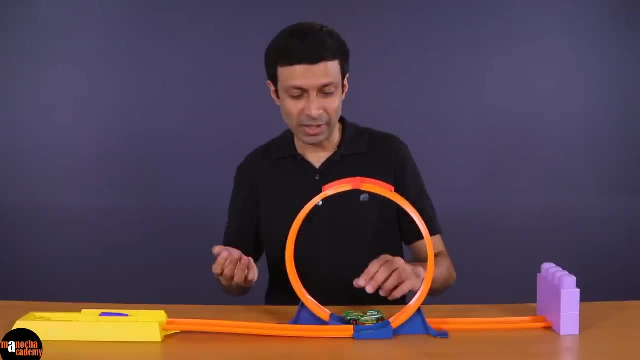 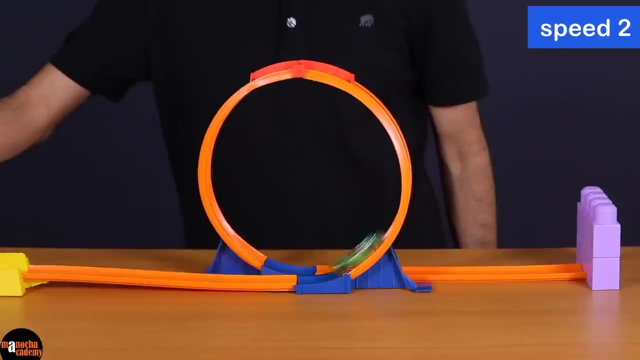 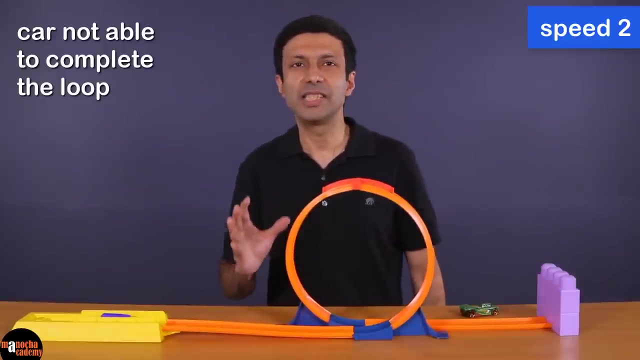 slow motion replay. it stops here. Now let's increase the speed to the next level. Again, the car is not able to complete the loop at this second speed. As you can see from the slow motion replay, the car falls off near the top of the loop. 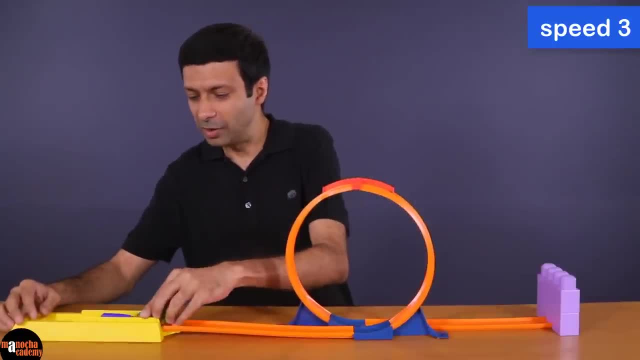 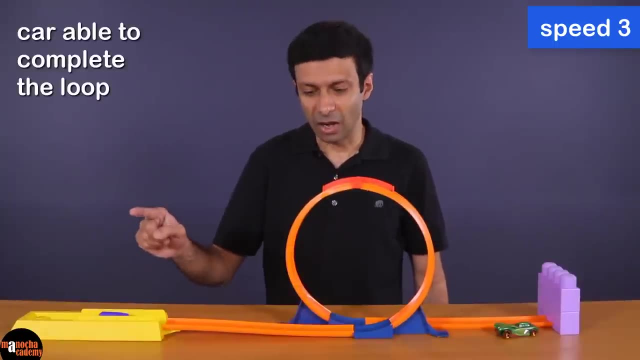 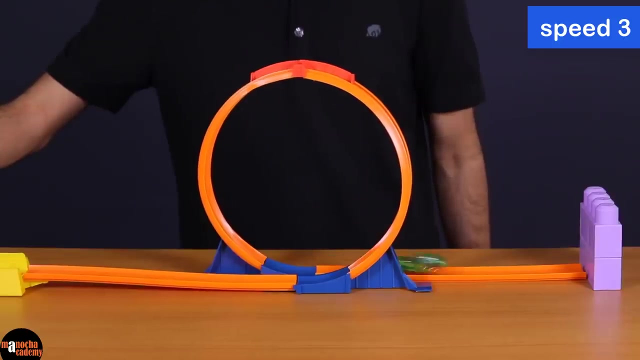 Now let's go ahead and increase the speed to the third level. So at the third speed the car is able to complete the loop. Here's the slow motion replay for you. Now let's increase the speed of the car to the fourth level, the highest speed. 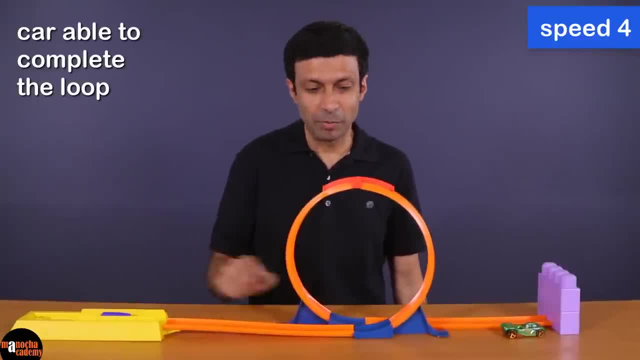 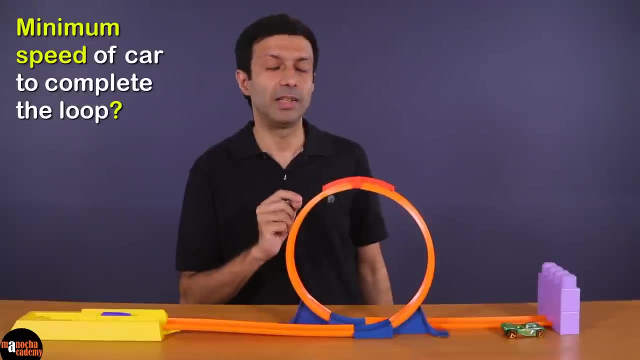 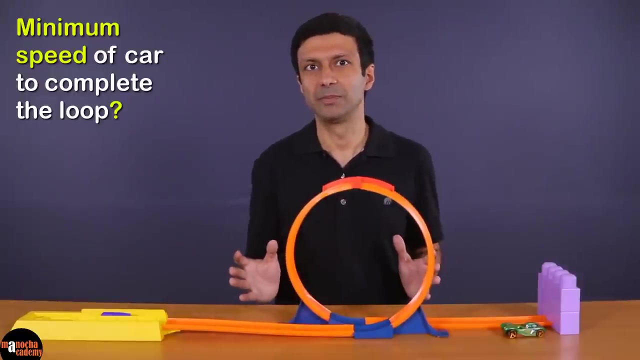 As expected, at the highest speed, the car is able to complete the loop comfortably. Now an interesting question is: what is the minimum speed needed for the car to be able to complete the loop? How can we calculate the minimum speed? We can take the help of the law of conservation of energy. 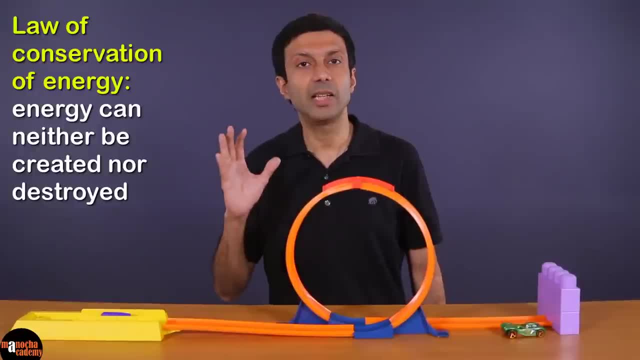 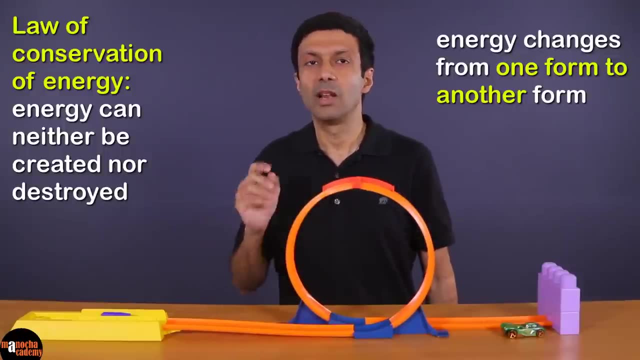 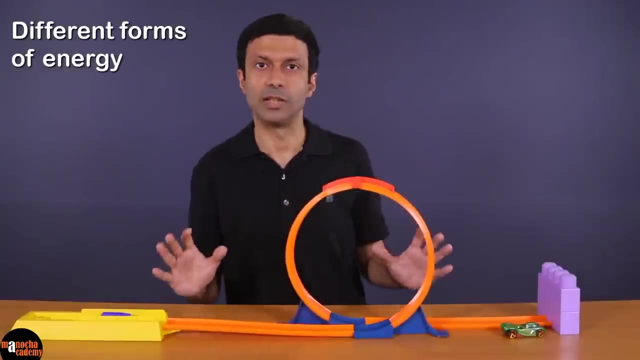 The law of conservation of energy states that energy can neither be created nor destroyed. Energy changes from one form to another form. Now, before we can use the law of conservation of energy here, let's take a look at the different forms of energy that are involved here. 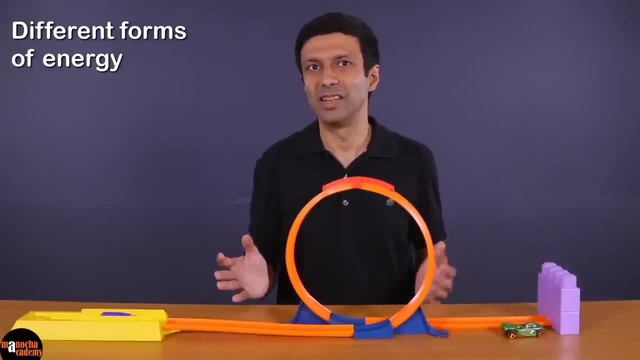 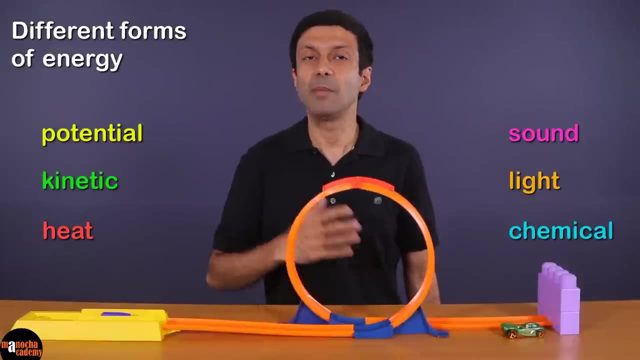 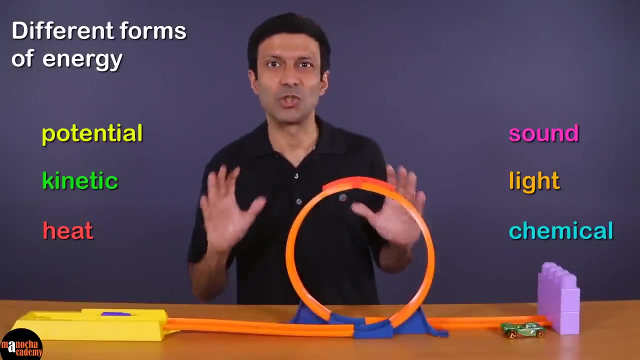 I'm sure you've heard that there are many different forms of energy, Such as potential energy, kinetic energy, heat energy, sound energy, light energy, chemical energy and so on. So what do you think? What forms of energy are involved in this toy? Let's analyze. 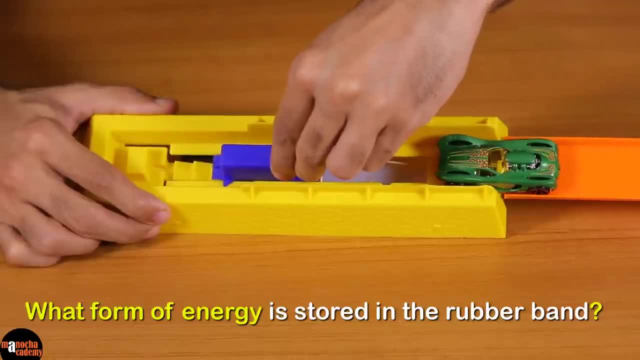 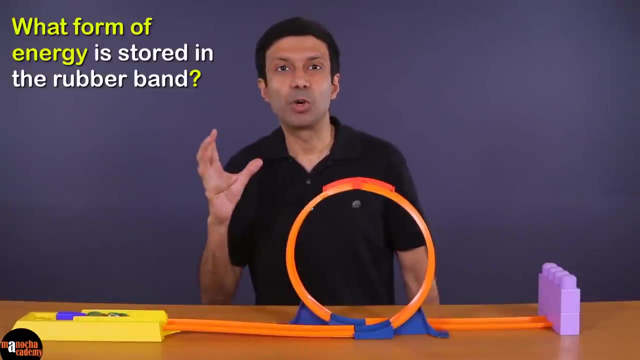 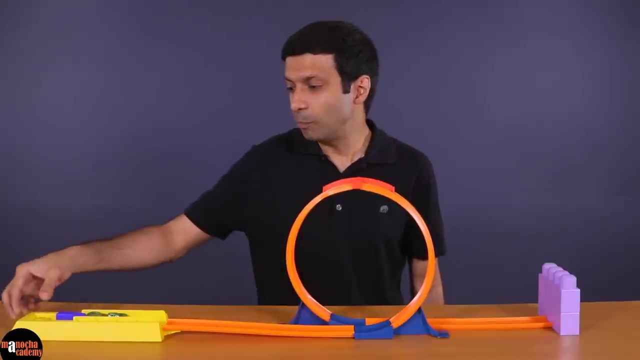 Now, when I pull this launcher, what form of energy is stored in the rubber band? That's right. the stretch rubber band has potential energy stored in it, Or, to be more specific, elastic potential energy. Now, when I press the launcher button, the rubber band gets released. 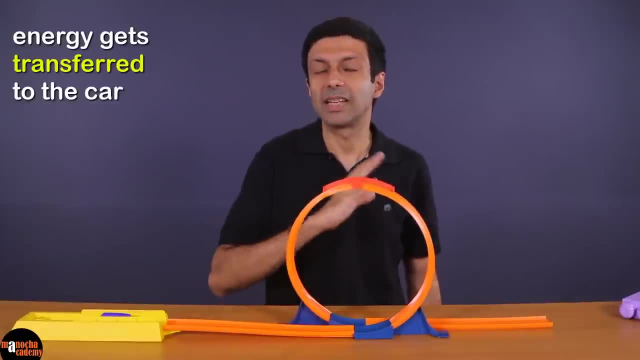 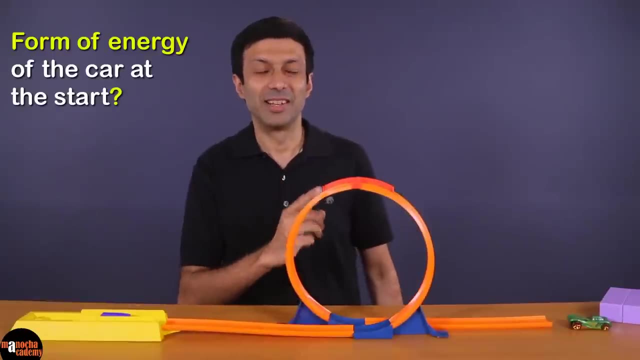 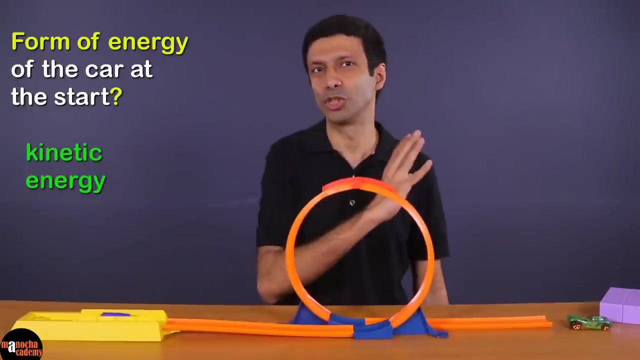 And the elastic potential energy of the rubber band gets transferred to the car. What form of energy does the car have at the start? That's right. the car is in motion, So the car has kinetic energy. Kinetic energy is the energy in motion. 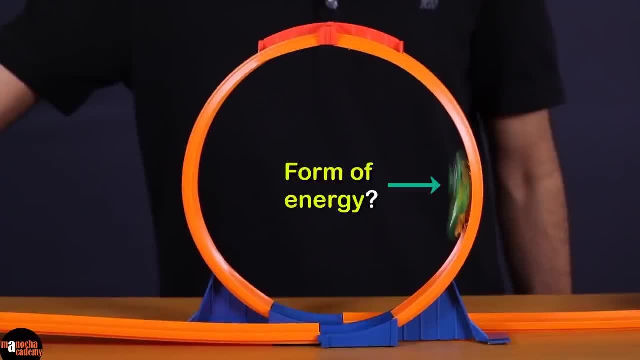 Now, as the moving car goes into motion, what form of energy does the car have at the start? That's right. the car has both potential and kinetic energy. Since the car is at a height from the table surface, it has gravitational potential energy. 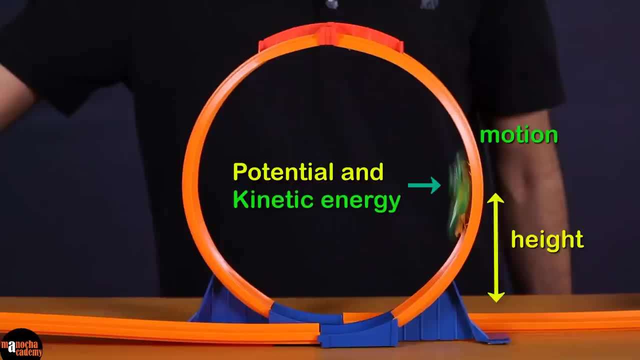 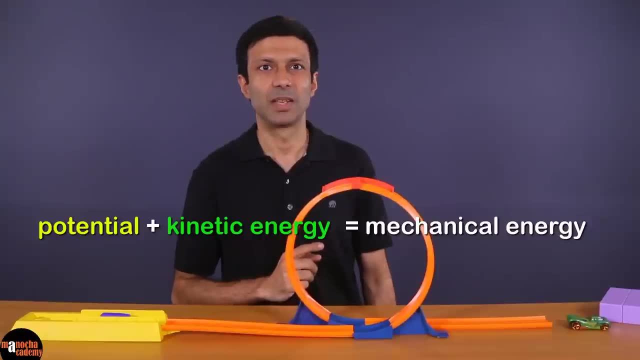 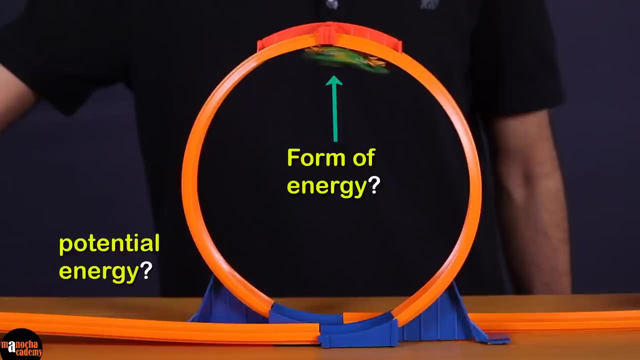 The car is also in motion, so it also has kinetic energy. The sum of potential and kinetic energy is known as mechanical energy. Now what happens when the car reaches the top of the loop? What form of energy does it have? Is it just potential energy, or potential energy and kinetic energy? 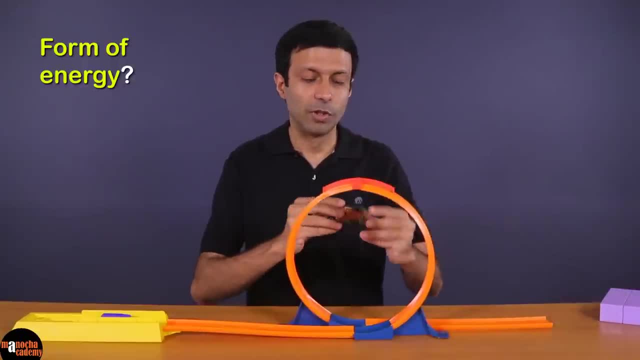 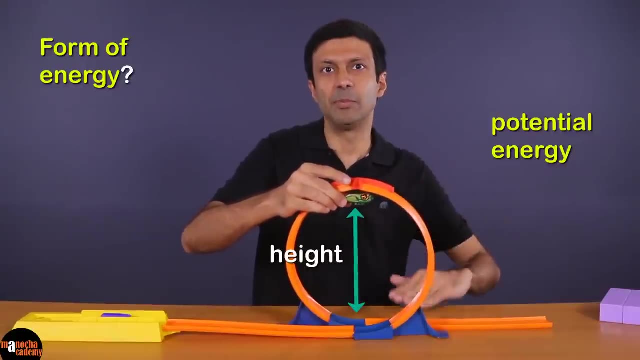 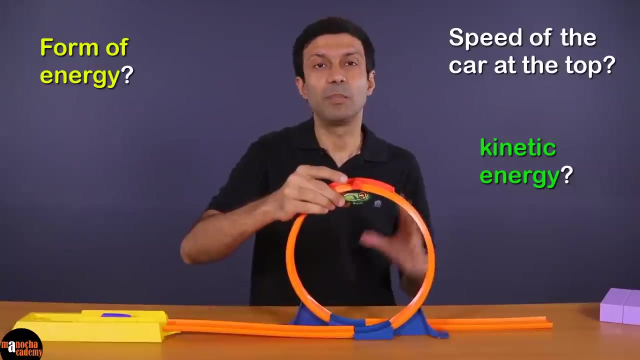 Now, this is a tricky one. So when the car is at the top of the loop, it definitely has potential energy Because it's at a height from the table surface. Now, what do you think about the kinetic energy here? Can the speed of the car be zero at the top? 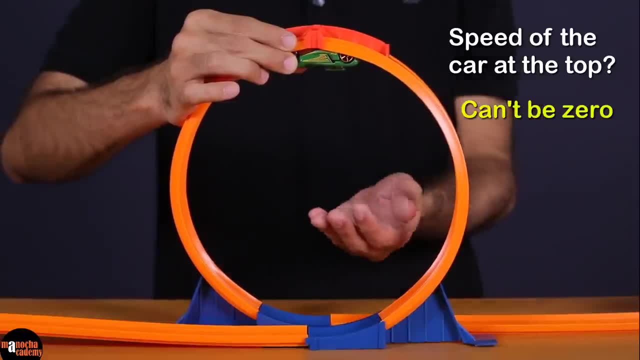 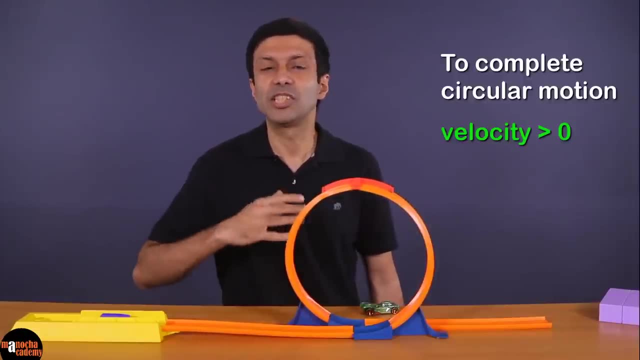 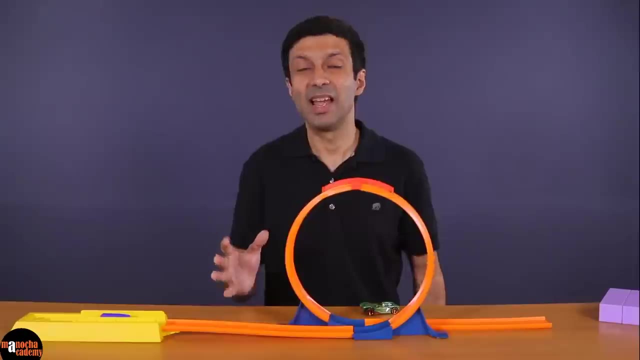 No, If the speed at the top was zero, then the car would just fall off. To complete the circular motion the car needs to have some speed, some velocity which is greater than zero. So at the top of the loop the car has both potential and kinetic energy. 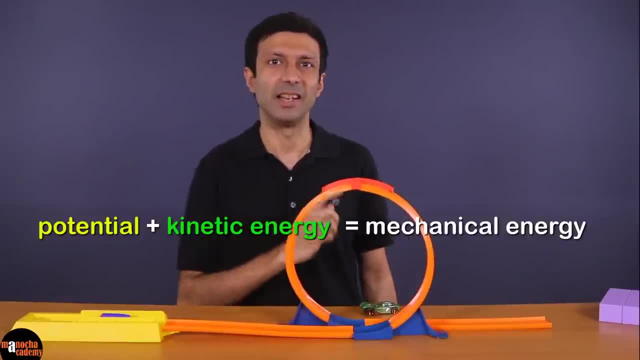 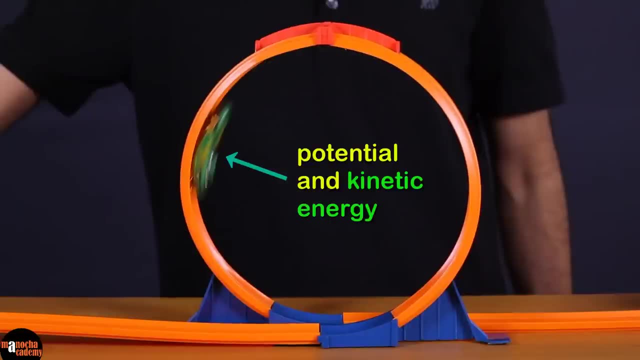 And the sum of potential and kinetic energy is known as mechanical energy. Now, as the car continues down the loop, the car has both potential and kinetic energy. So if the car exits the loop, what form of energy does it have? That's right, the car only has kinetic energy here. 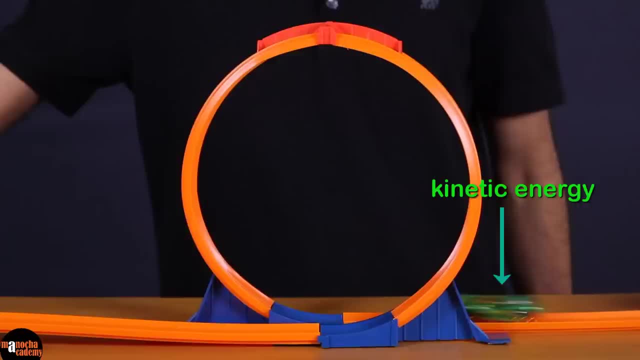 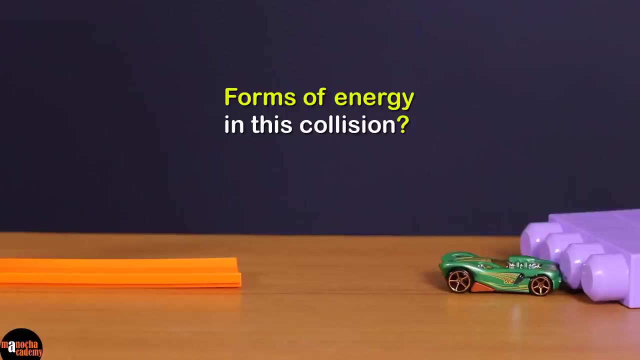 Since the car is not at a height, the potential energy is zero. So the car only has energy due to its motion, which is kinetic energy. And when the car finally hits the block and comes to a stop, what forms of energy are involved in this collision? 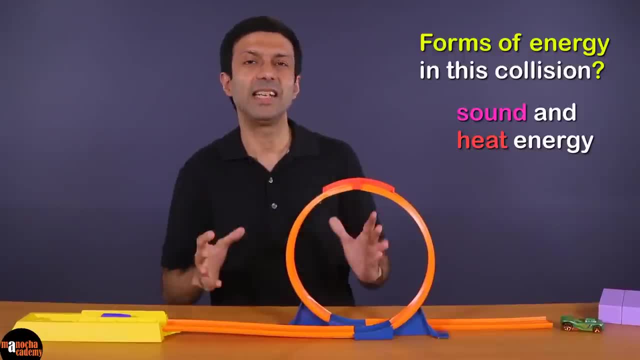 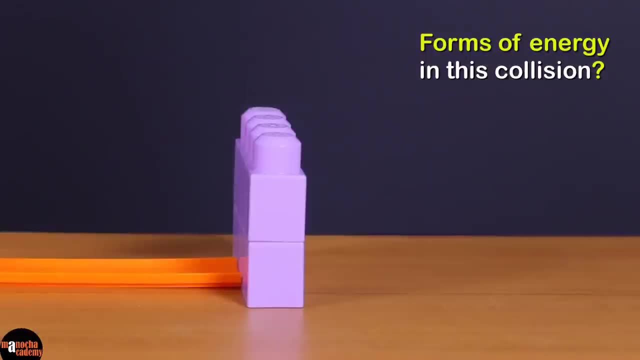 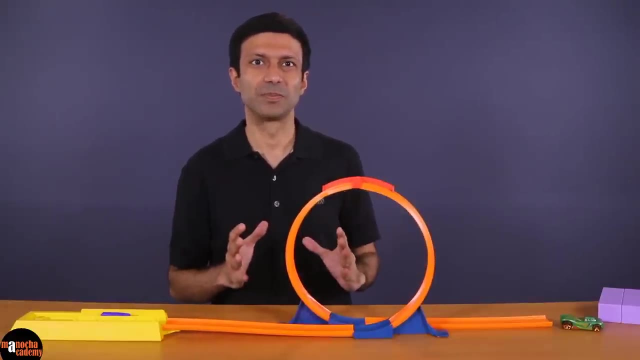 The collision of the car and the block produces sound and heat energy, And some of the kinetic energy of the car was transferred to the block. Did you hear the sound of the collision? And when two things collide, some heat is also produced. 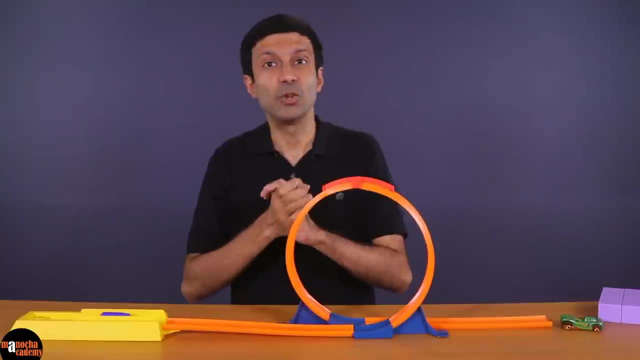 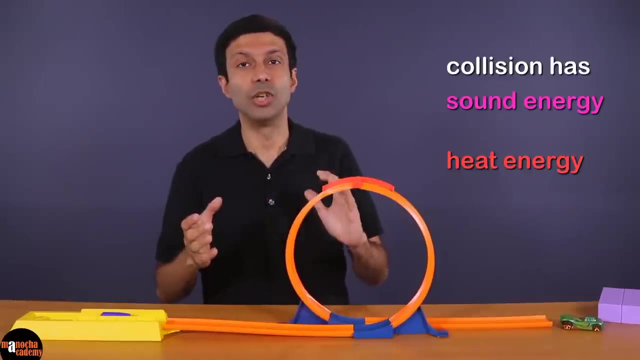 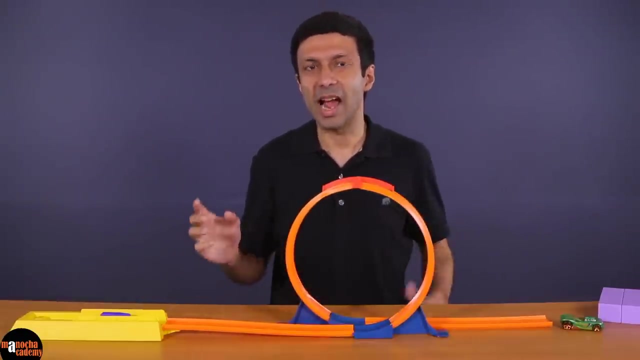 For example, try clapping your hands like this: Can you hear the sound energy And can you also feel the small heat energy generated in your hands. A collision usually has both sound and heat energy, So we have looked at the different forms of energy at different points in the journey of this car. 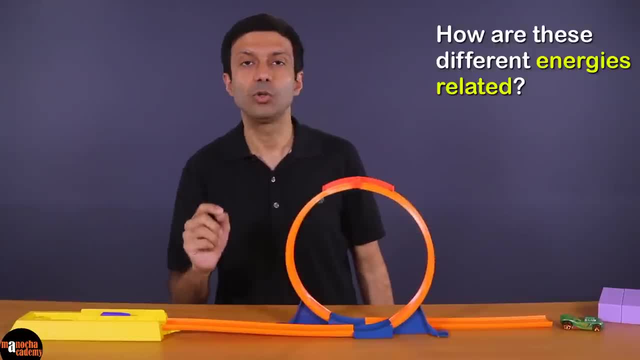 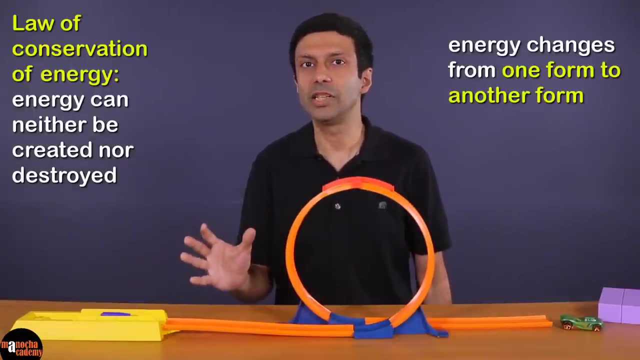 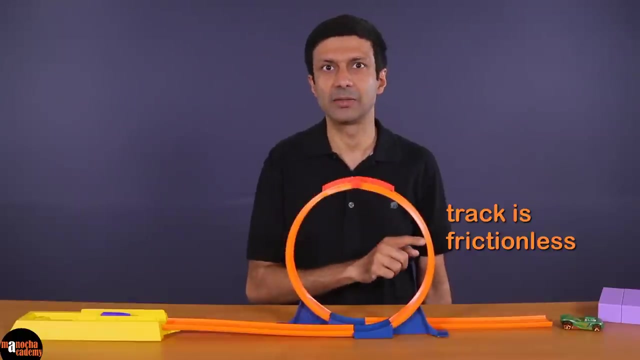 Now, how are these different energies related? According to the law of conservation of energy, energy can neither be created nor destroyed. Energy changes from one form to another form. Now let's assume that this track is frictionless, So no energy is lost due to friction. 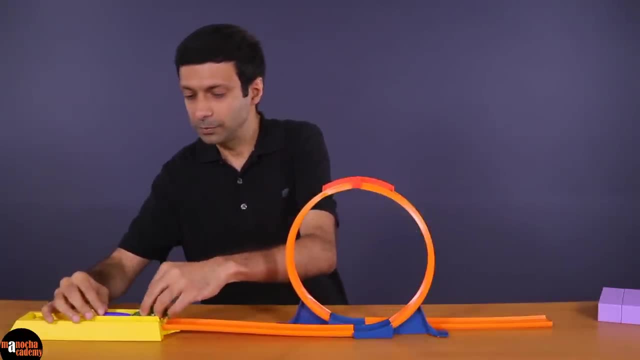 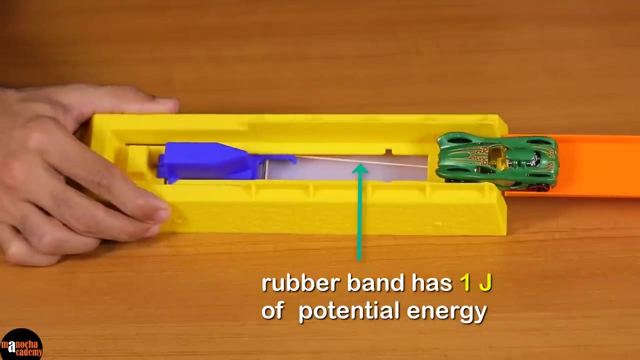 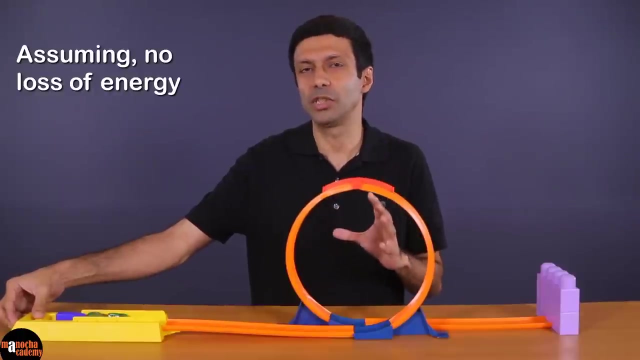 And now let's say, when this launcher is pulled, the rubber band stores one joule of potential energy in it, Assuming there is no loss of energy. now, when I press this launcher, according to the law of conservation of energy, all the elastic potential energy of the rubber band is going to get transferred to the car. 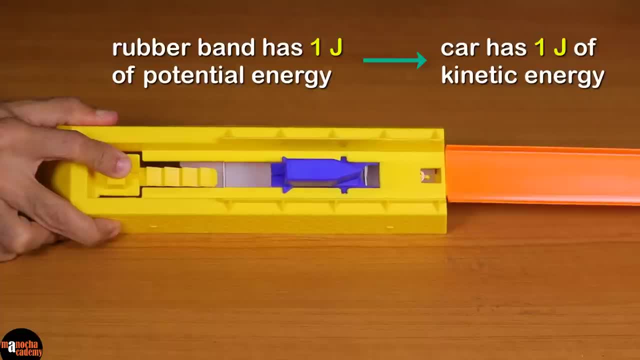 So the car now has one joule of kinetic energy. Actually, when the launcher hits the block, the rubber band is going to get transferred to the car, So the car now has one joule of kinetic energy. When the launcher hits the car, some of the energy gets converted into sound and heat energy. 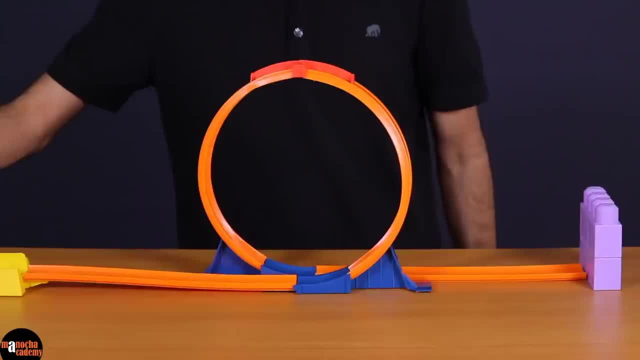 But just to keep things simple, we'll ignore it. As the car enters the loop, some of the kinetic energy gets converted into potential energy, But the sum of the potential and kinetic energy of the car, which is the mechanical energy, will still be one joule. 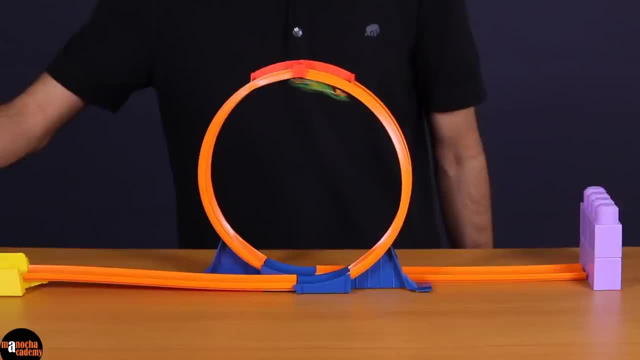 As the car reaches the top, the potential energy of the car increases, but the kinetic energy decreases Again. the sum of the potential energy and kinetic energy, that is, the mechanical energy, is one joule. The same applies when the car comes down the loop. 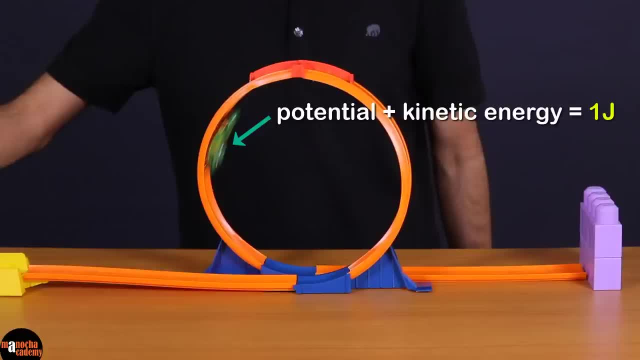 Potential energy decreases and kinetic energy increases. And when the car exits the loop, how much energy does it have? That's right, one joule. And when the car collides with the block, sound and heat energy is produced by the collision. 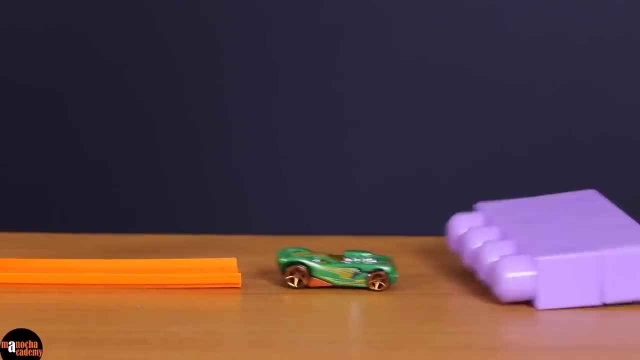 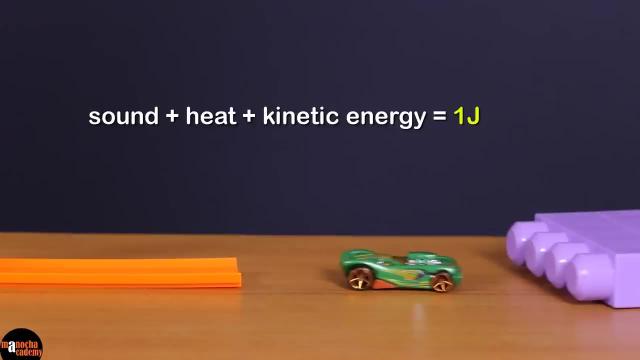 And some of the kinetic energy of the car is transferred to the block. So the sum of the sound and heat energy of the collision and the kinetic energy of the block is equal to one joule. This is the law of conservation of energy. The amount of energy is conserved. 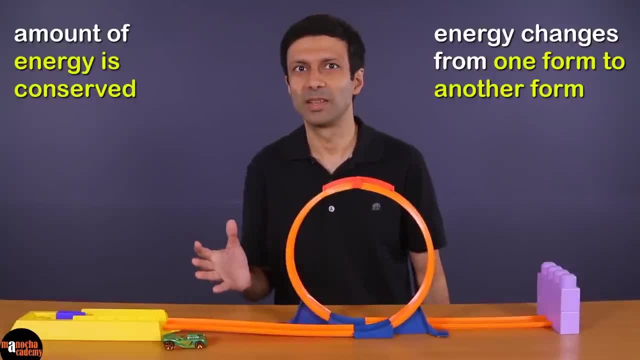 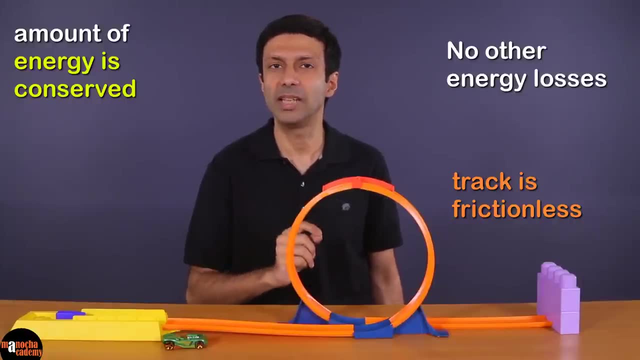 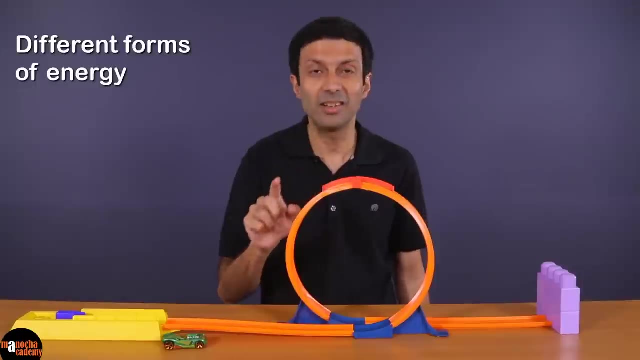 But energy changes from one form to another form. Of course, we assume that the track is frictionless And there are no other energy losses in the form of heat and sound. This is the law of sound energy. Now that we've looked at the different forms of energy at different points in the car's, 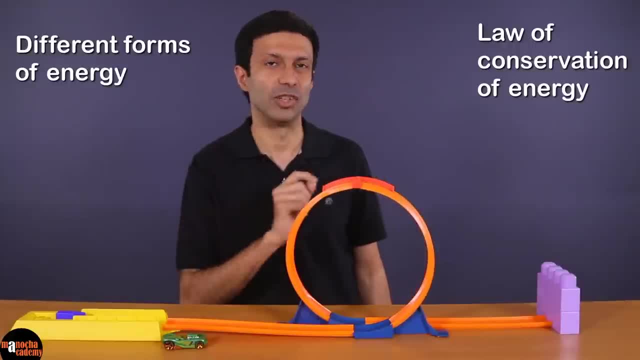 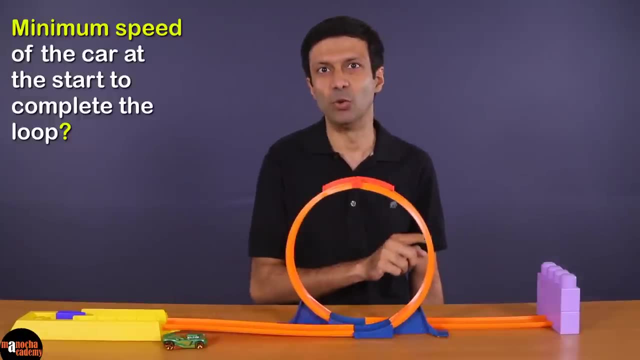 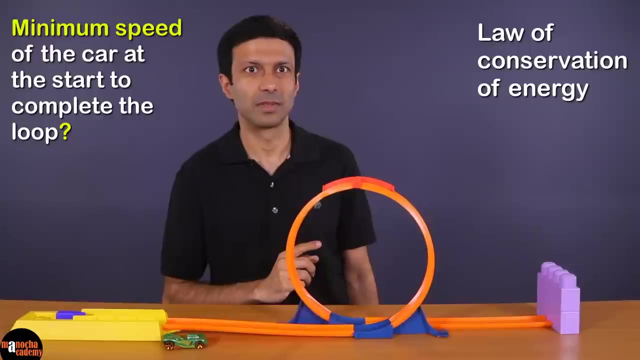 journey and the law of conservation of energy. let's go back to our question: What should be the minimum speed of the car at the start so that it can complete the loop? So let's see how we can apply the law of conservation of energy to solve this question. 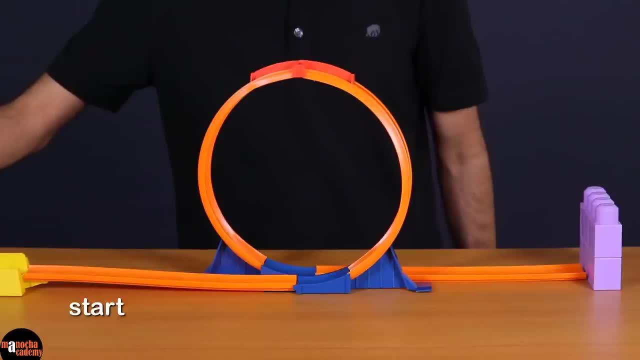 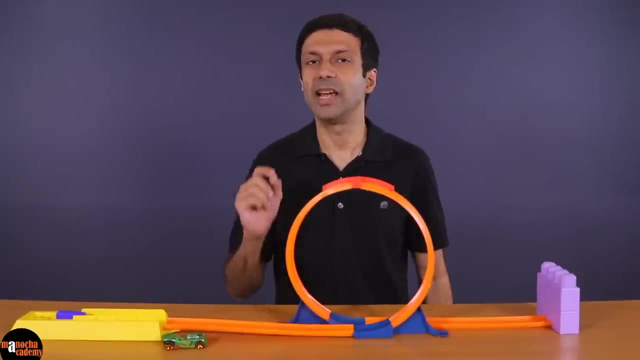 The two points that we are interested in, which the car starts off and then the point where the car is at the top of the loop. According to the law of conservation of energy, the energy of the car at the start is exactly equal to the energy of the car at the top of the loop. 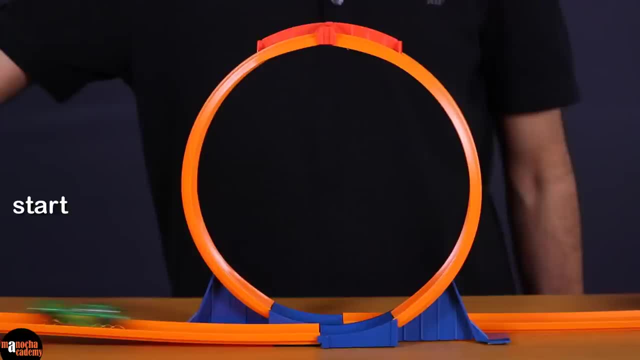 What was the energy of the car at the start? That's right: kinetic energy. The kinetic energy formula is half m- v square, where m is the mass of the car and v is the velocity. If we take the velocity at the start as v1, the kinetic energy at the start is half m- v1. 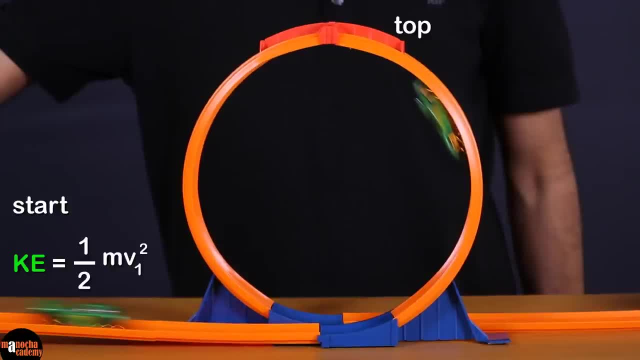 square, And the energy of the car at the top of the loop is both potential and kinetic energy. When the car is at the top of the loop, the potential energy equals m, g, h2.. Here m is the mass of the car, g is the acceleration due to gravity and h2 is the height of the car. 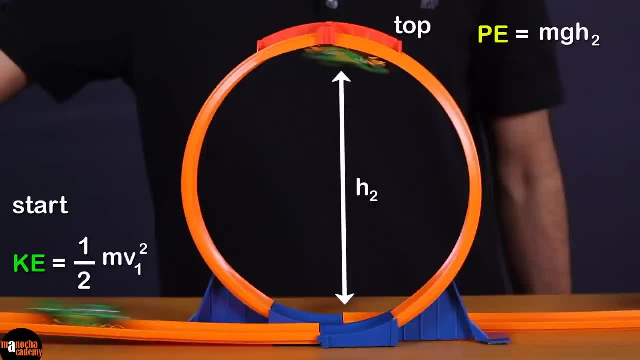 And if we take the velocity of the car at the top of the loop as v2, then the kinetic energy at the top of the loop will be half m v2 square. As we discussed, the energy of the car at the start equals the energy of the car at the top of the loop. 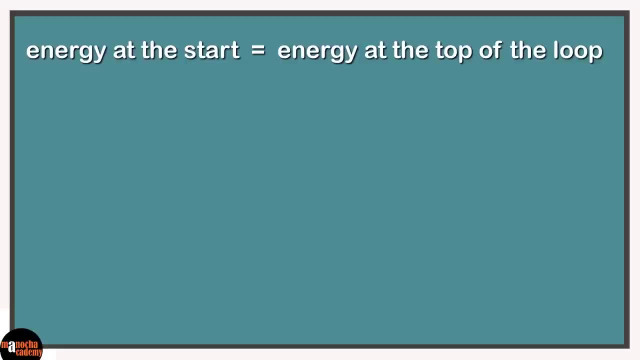 Let's plug in these formulas into our equation and we get: half m v1 square equals m g h2 plus half m v2 square. The mass of the car gets cancelled, So actually the mass of the car doesn't matter. We are now left with half m v1 square equals m g h2, plus half m v2 square. 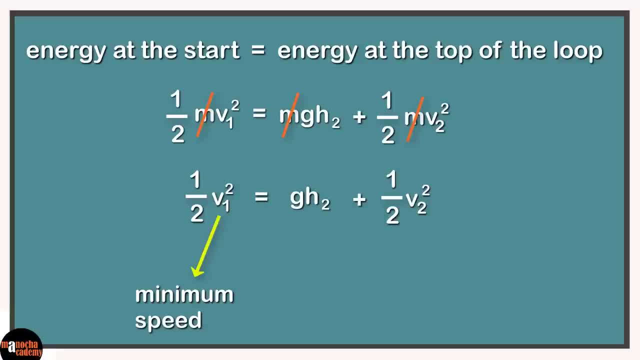 We need to calculate v1, the minimum speed of the car to complete the loop. Let us take the value of acceleration due to gravity g as 9.8 m per second square. We need h2, the height of the loop and the whole velocity at the top of the loop. Let us take the value of the acceleration due to gravity g as 9.8 m per second square. We need h2, the height of the loop. We need h2, the height of the loop. So let's use thisander to deduce��ело. 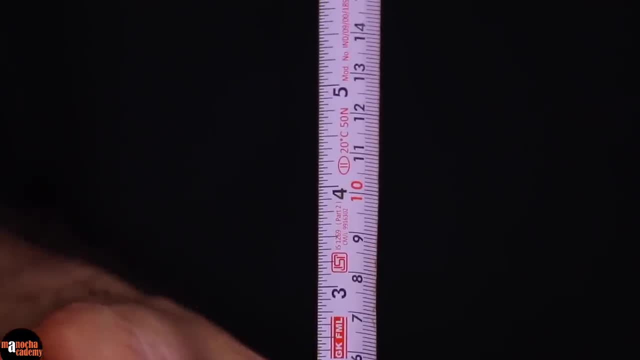 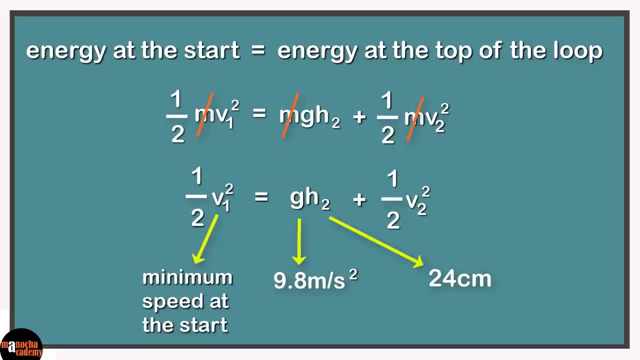 tape to measure the height of the loop from the table surface. As you can see, the height is 24 cm. Let's convert it into SI units, So H2 is 0.24 m. But how do we calculate V2, the velocity of the car at the top of the loop? 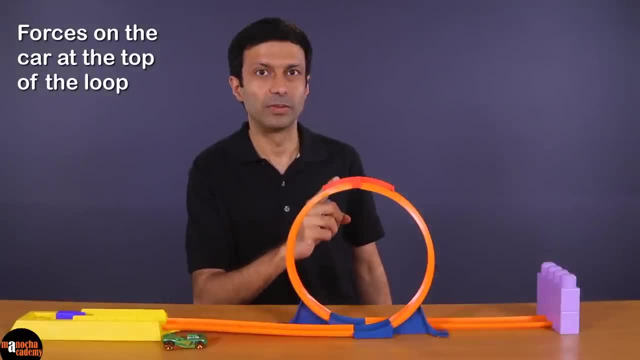 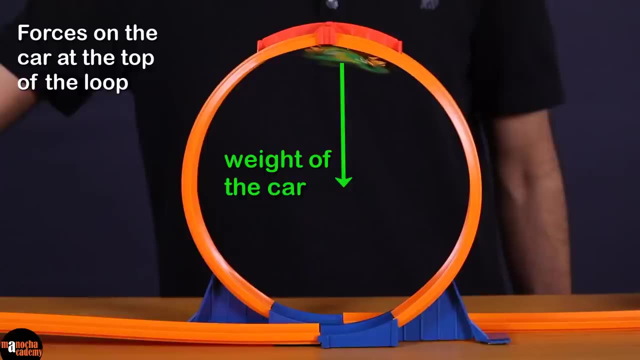 We need to analyze the forces on the car at the top of the loop. When the car is at the top of the loop, the weight of the car is acting downwards. There is also the normal reaction by the track on the car. The normal reaction is also downwards at the top. 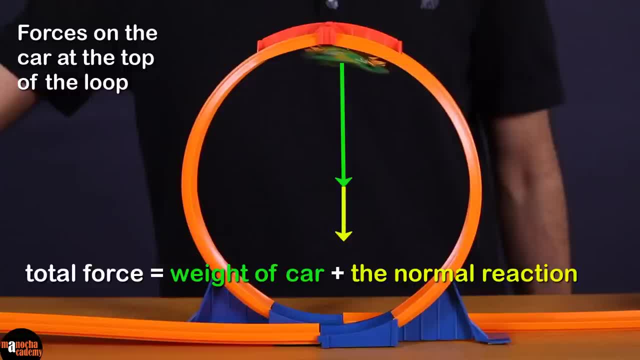 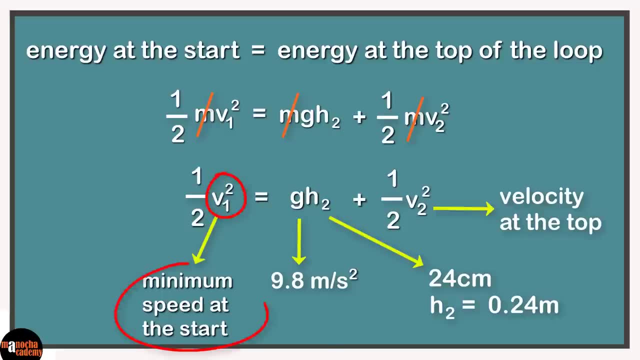 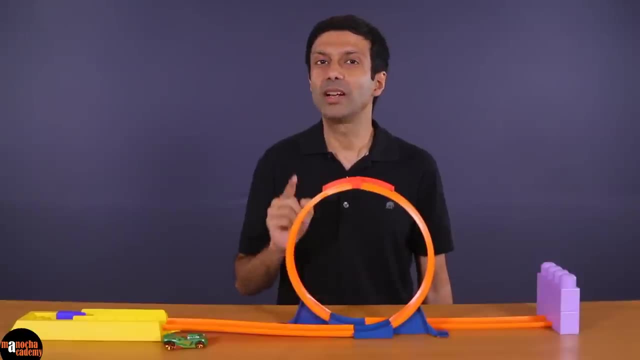 So the total force on the car at the top of the loop is the weight plus the normal reaction. Remember, we want to find V1, the minimum speed of the car at the start, so that it is able to complete the loop. Now, when the car starts off at this minimum speed and then it reaches the top, it is almost. 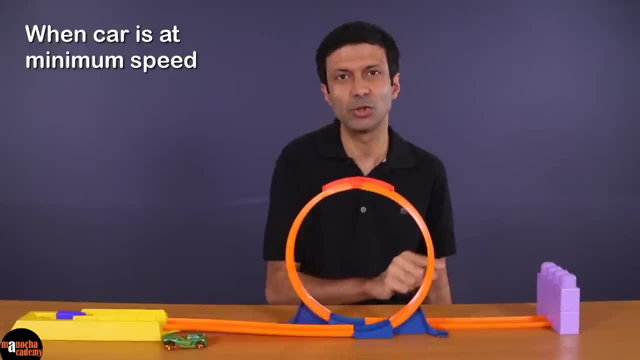 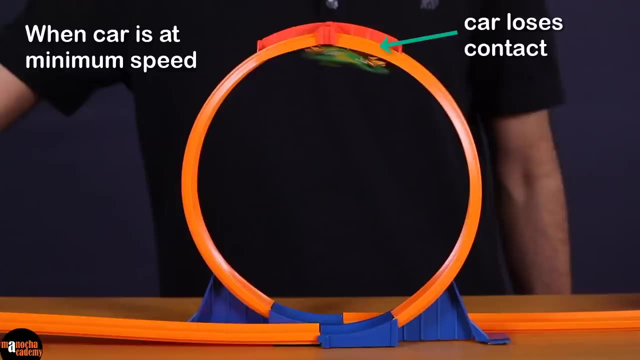 about to fall and it just barely manages to complete the loop. In this special case, when the car is at the top of the loop, the car will just lose contact with the track and is about to fall. So the normal reaction is equal to zero and the weight of the car is the only force acting. 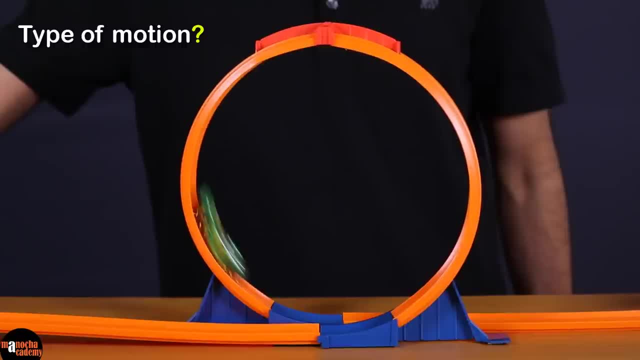 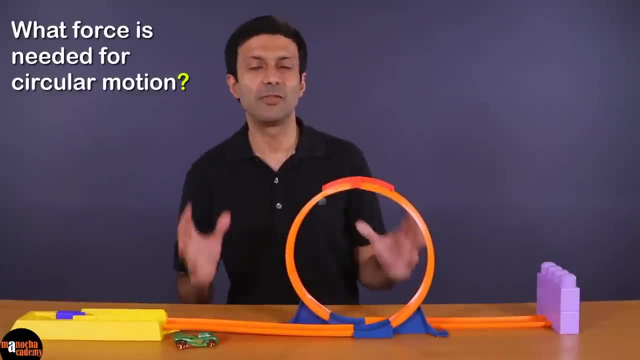 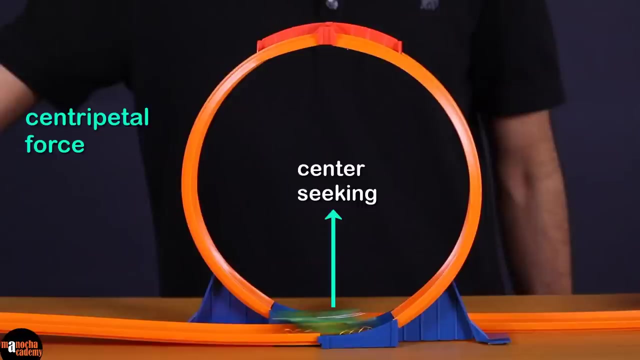 on it. What kind of motion is the car in when it goes around the loop? In this loop, the car is in circular motion. What kind of force is needed for circular motion? That's right, centripetal force. The word centripetal means centre-seeking. 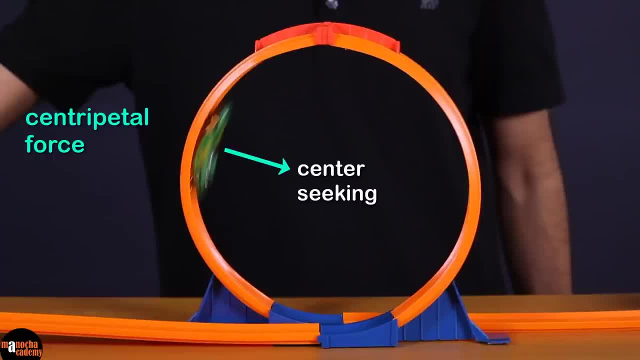 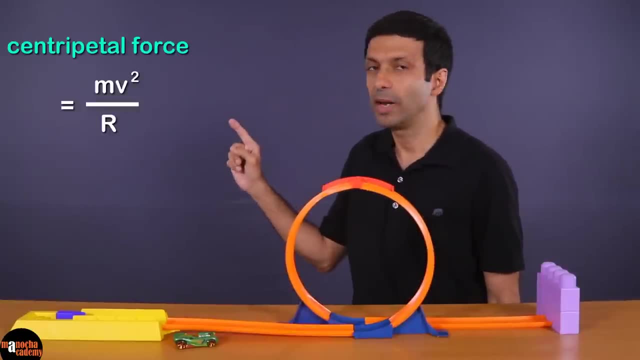 So in the loop the car experiences a centripetal force. What is the formula of centripetal force? The formula of this force is MV2 by V1.. The formula of this force is MV2 by V1.. The formula of this force is MV2 by V1.. 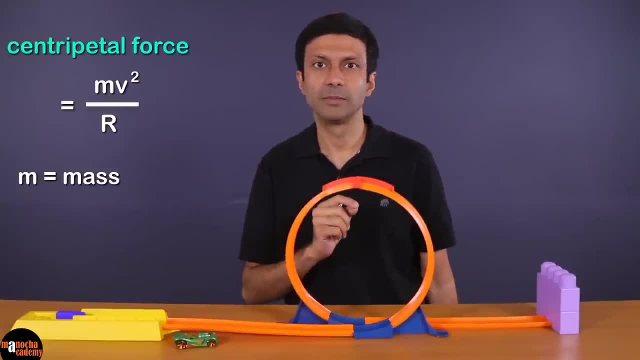 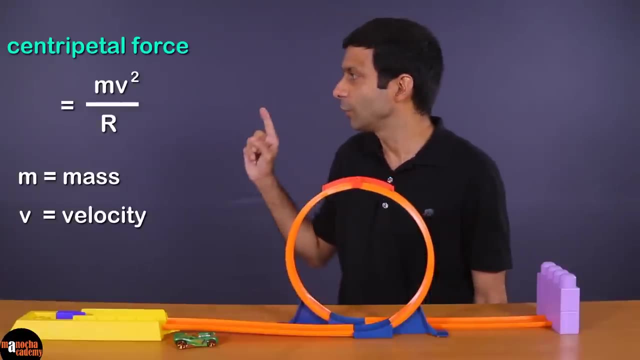 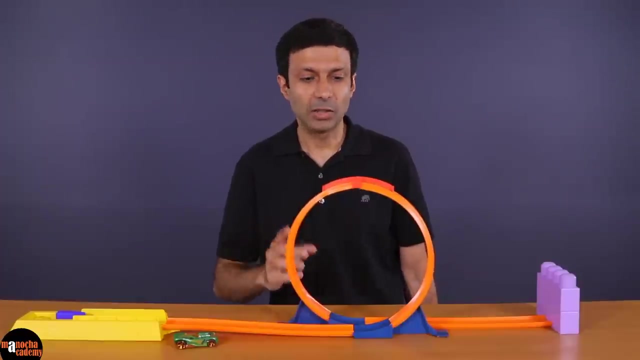 The formula of this force is MV2 by R, where M is the mass of the body and V2 by R is the centripetal acceleration. V is the velocity of the body here and R is the radius of this circle. Now, as we saw at the top of the loop, the only force is the weight of the car, since 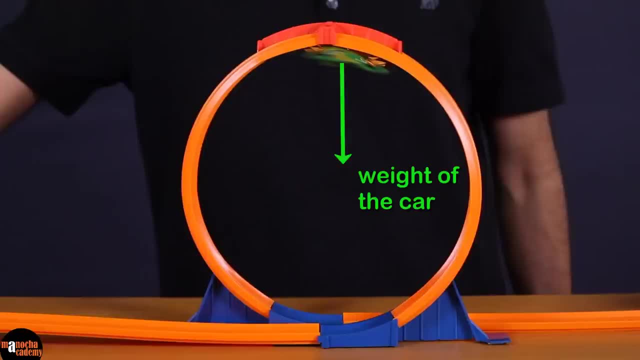 normal reaction is zero at the top. So weight is the centripetal force acting on the car making it go in a circular motion. So weight is the centripetal force acting on the car making it go in a circular motion. We can say at the top, centripetal force equals the weight. 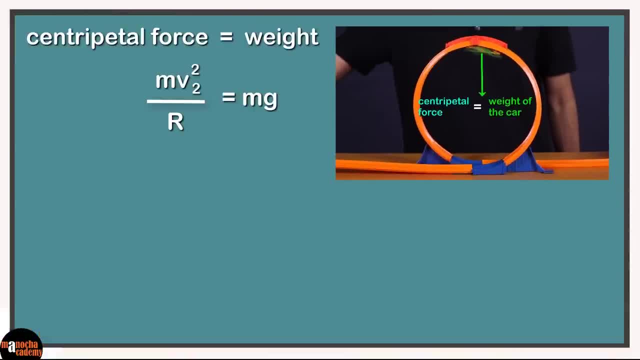 Let's use the formula of centripetal force. so we get MV2 square by R is equal to MG, the weight, The mass cancels, and we have V2 square equal to GR. So V2, the velocity at the top, is square root of GR. 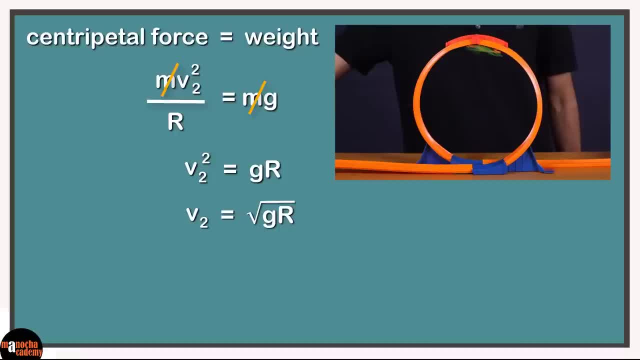 Now let's go and substitute V2. in a square, The weight of the car is equal to GR. So that's the formula of V2 square by R. That's, V2 square by R equals Mg. We need to subtract V2's weight. 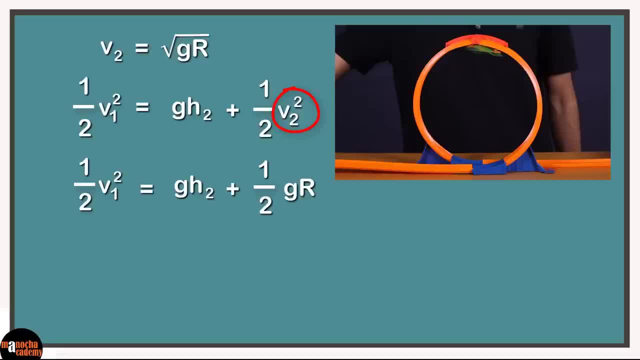 So that's Mg, our main equation. We get half V1 square, equal to GH2, plus half GR R. the radius of the loop will be the diameter by 2, which is the height- H2 that we measured divided by 2.. Substituting: 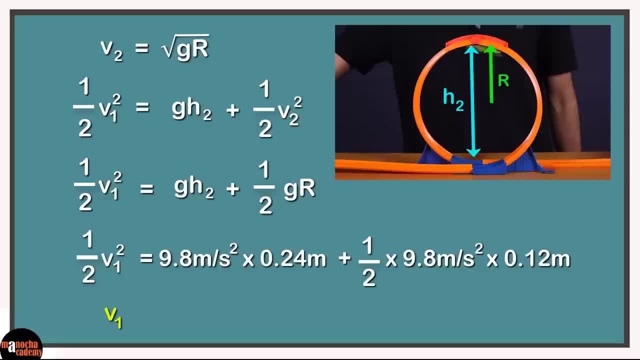 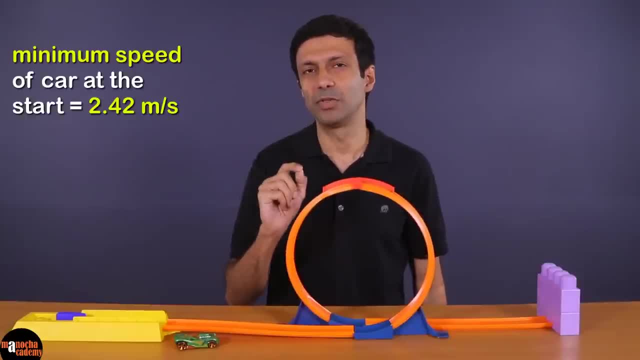 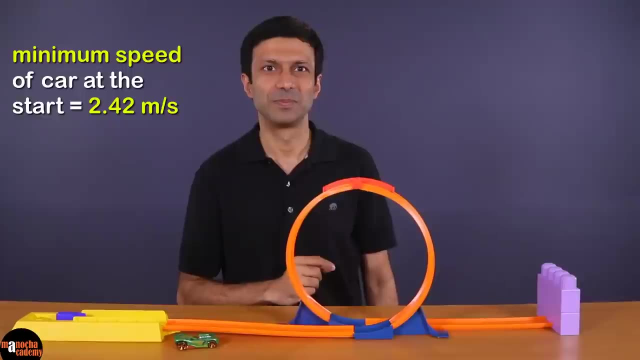 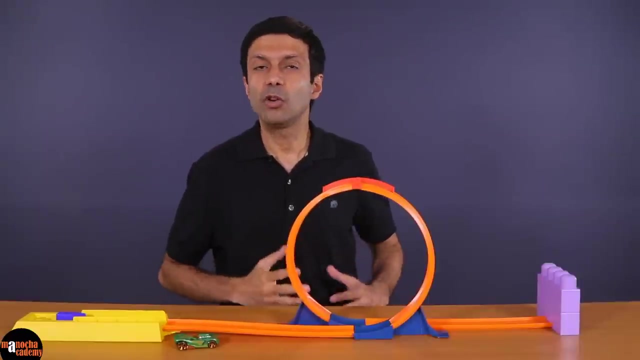 all the values and solving, we get V1 equal to 2.42 meter per second. As we calculated, the minimum speed of the car at the start to complete the loop is 2.42 meter per second. I hope you enjoyed this video and the physics behind this toy is clear to you. Have you been?